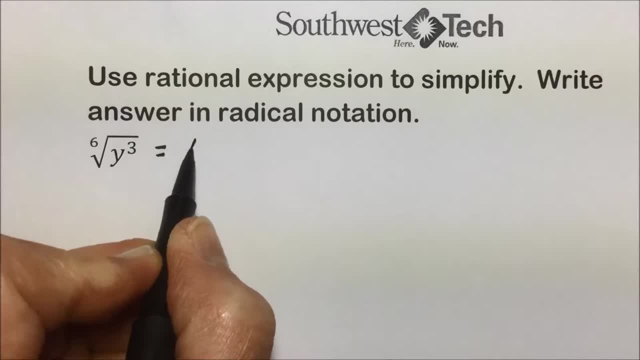 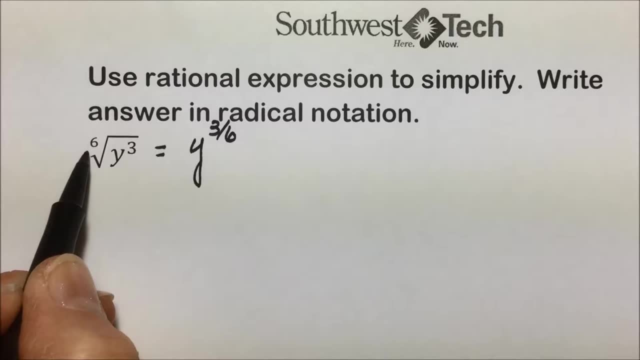 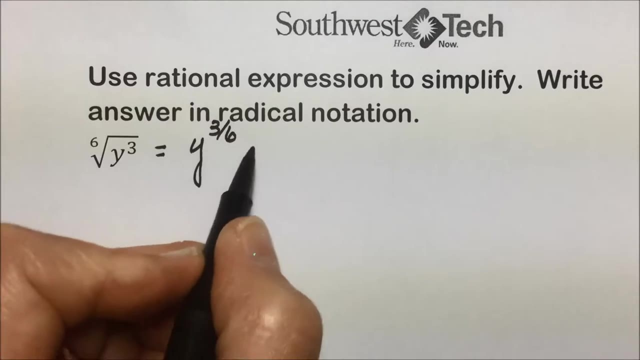 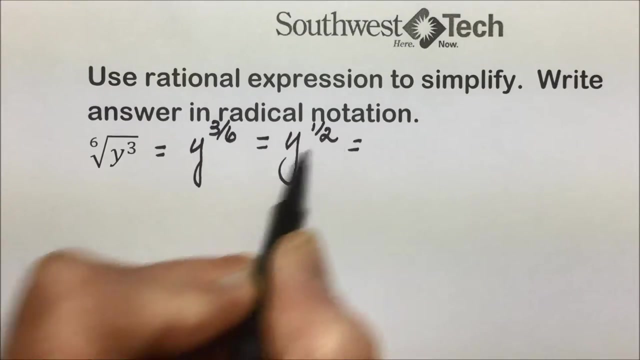 of our exponential power. So we will have y to the 3 over 6th power as a translation from this radical to a rational exponential power. Looking now at that rational power, 3 over 6th reduces to 1 half. and now that it's simplified, 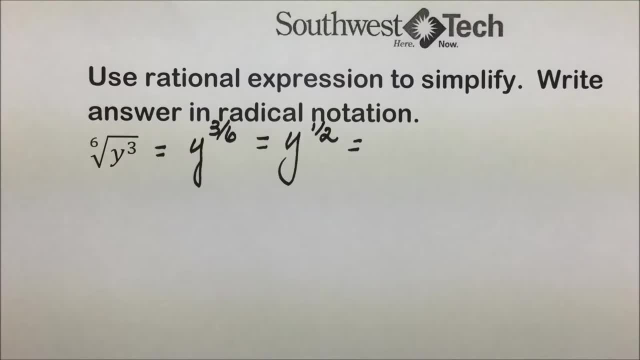 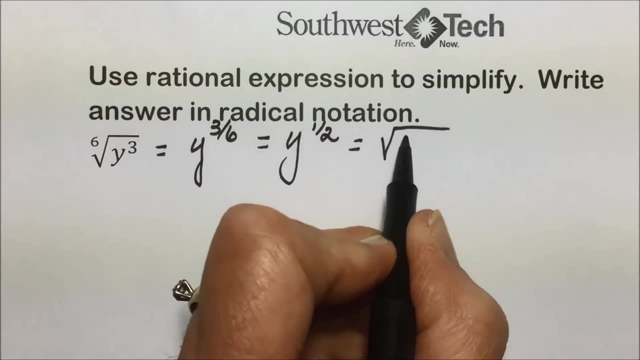 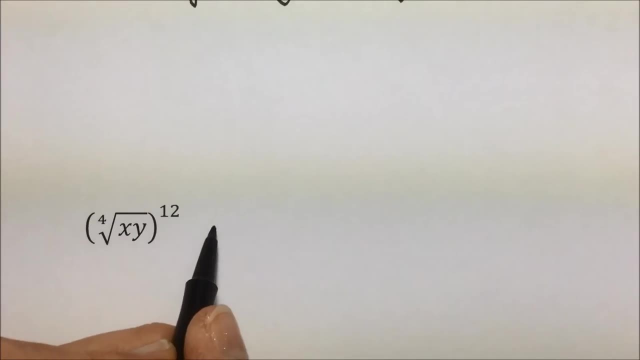 we'll put it back in radical notation. The denominator is the index on our radical, So it's the square root. Because there's no index, it's understood to be 2 of y. In this next problem, very similar, we have the quantity x, y. 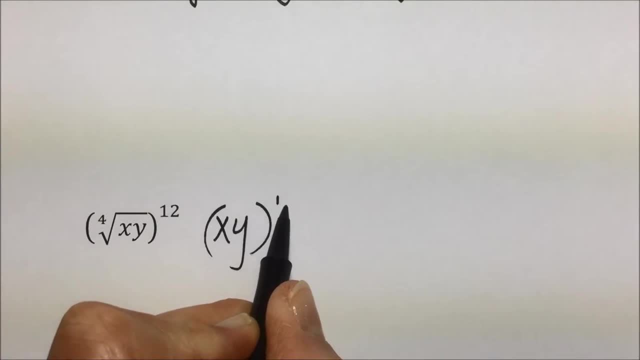 But in the case of this volt, like the one, we had the value of y, t, so we lose y And now we have x equal to y, t and y mais 2 e. 3 times 4, is 9, e to the 3rd power and 5 power is 12, 0,. 1st day. 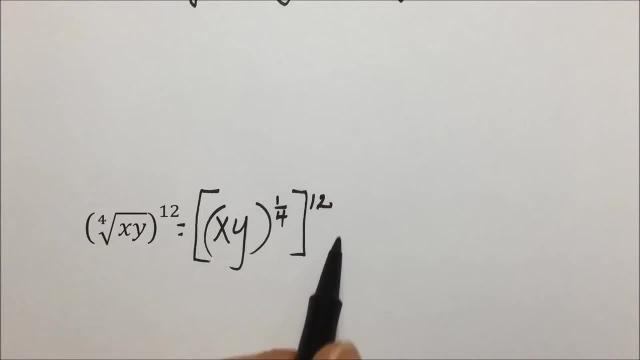 So if y is also inside a radius very similar to our original theta, we would have an x equal to y settlements with agreeing Fourier across every radius of the table. there we go. At least that's what we have in here. 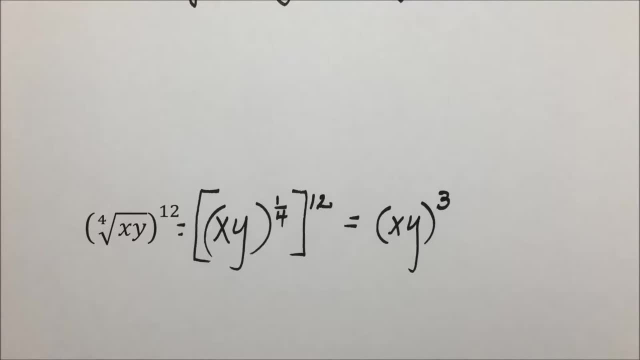 To the right. we take the Y. for the simplification of this, Our final answer is the quantity xy to the third, or we could raise each of these terms, in other words the product to the power. we could say the equivalent of x to the third times y to the third. 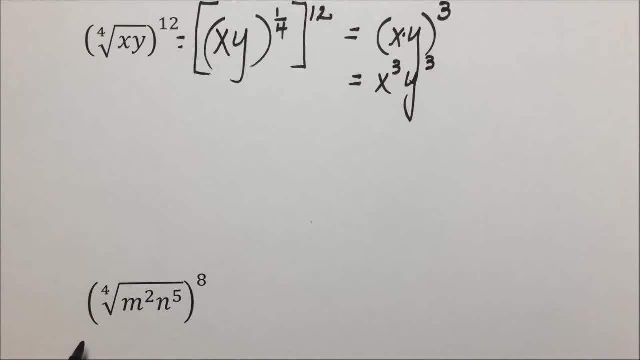 This next problem is asking us to simplify this rational expression. The radical is the fourth root of this quantity and then raised to the eighth power. So we have m to the second, n to the fifth. It's raised to the eighth but has the fourth root, which is the denominator. 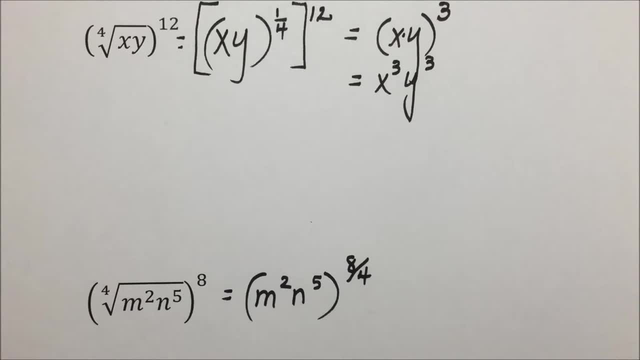 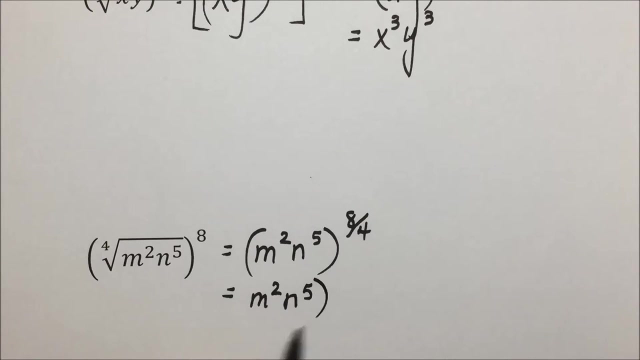 The index becomes the denominator of our rational expression, Similar to the last one we can do the division 8 divided by 4, as you can see, This means that this is equivalent to m, to the second, n to the fifth raised, to the. 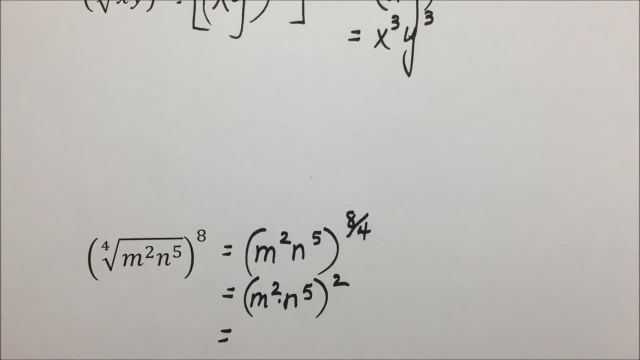 second power. Each of these terms, then, or factors, is raised to the second power, and our simplification would be: m to the second. raised to the second would be m to the fourth, n to the fifth, also raised to the second, will leave us with m to the tenth power. There, 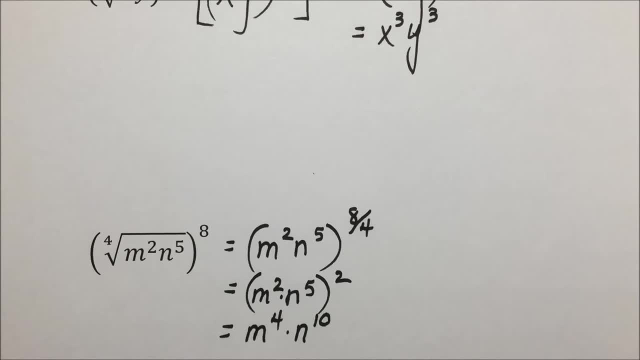 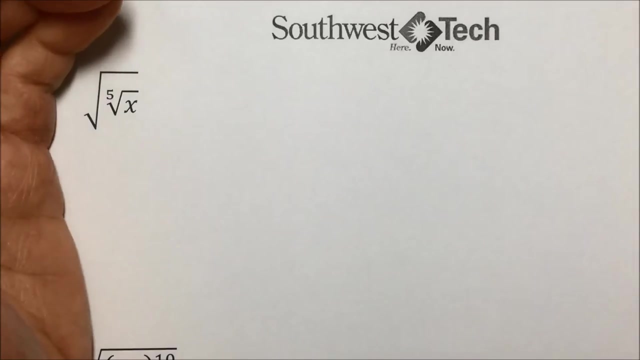 is no radical notation, But we have simplified the problem. In this next problem we have the fifth root of x and then, taking the square root of it and thinking about order of operations, we work from the innermost out, and so we have. 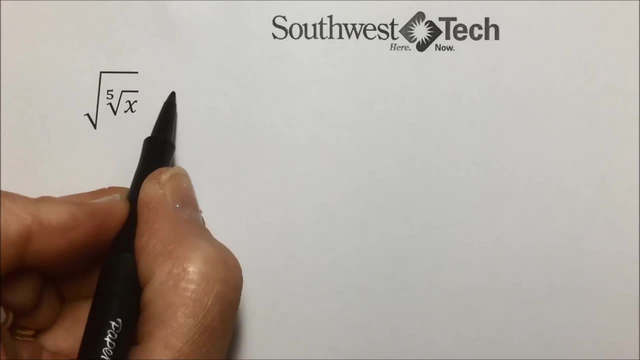 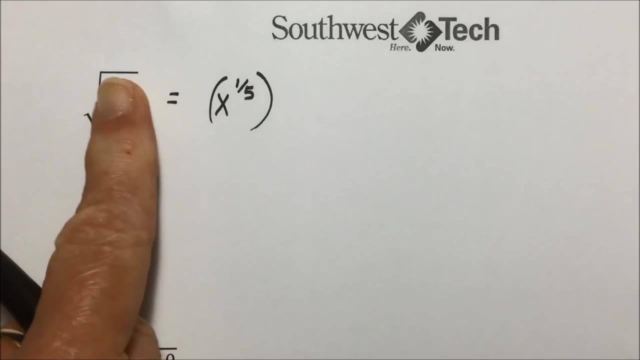 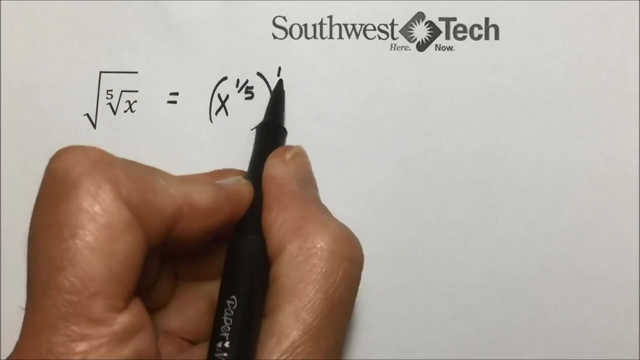 to replace this radical with a rational exponent. so the fifth root of x would be equivalent to x to the one-fifth, And then that is the square root of x. and then taking the square root of x and then having the square root of it, which in rational exponents means it would be that quantity. 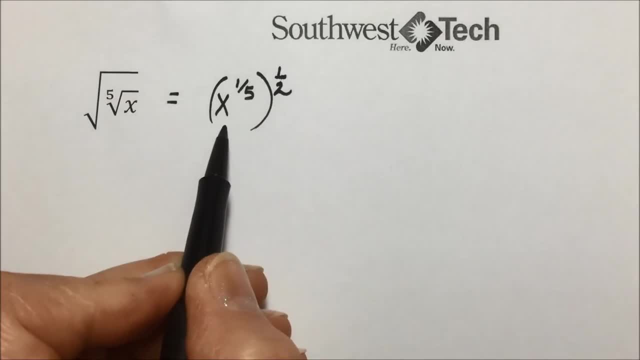 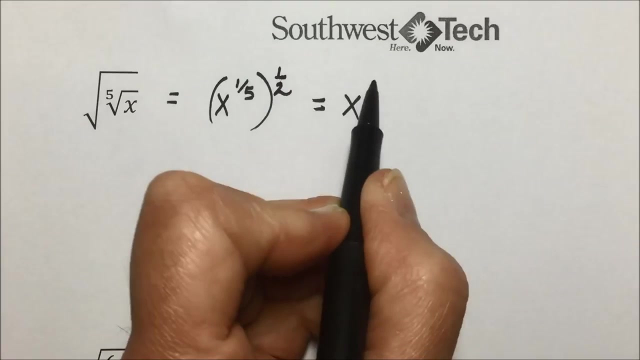 to the one-half power. Now that it's in exponential form, we can use our law of exponent: When we have a power raised to a power, we multiply those powers together. Multiplying numerators gives us 1,. multiplying denominators gives us 10.. 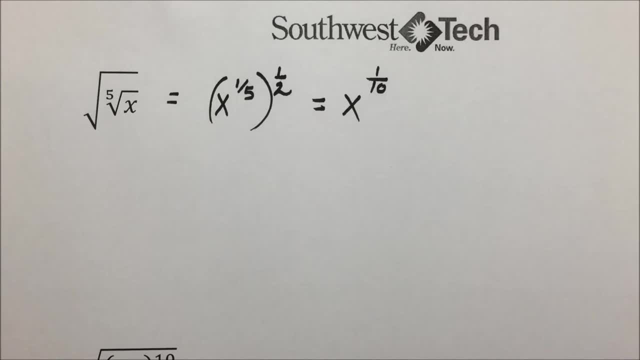 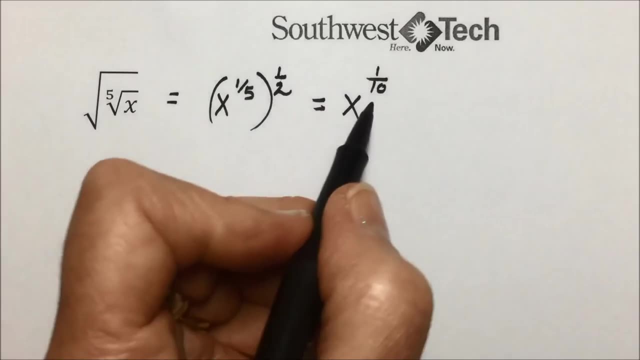 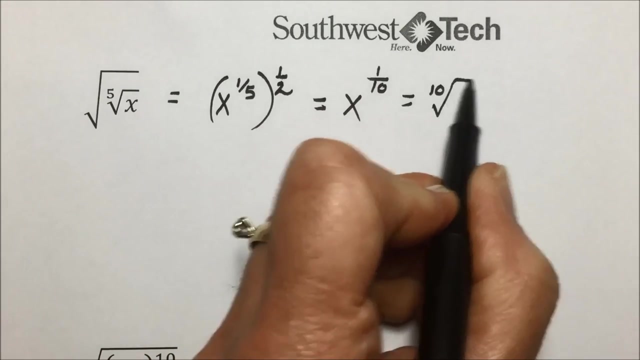 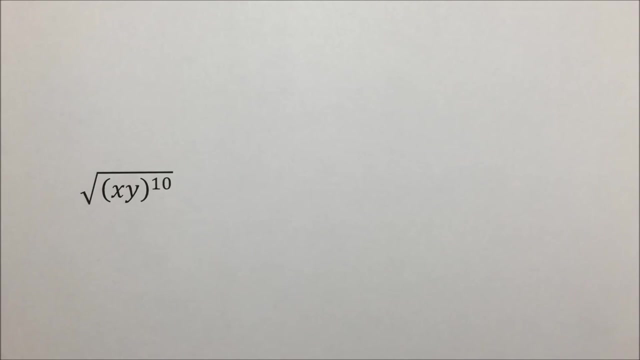 We've simplified, Going through exponential form, and now we need to convert it back to the radical notation. x to the one-tenth power means the equivalent of taking the tenth root of that quantity and in this case, x. In this last example, we are taking the square root of this quantity, the radicand, which. 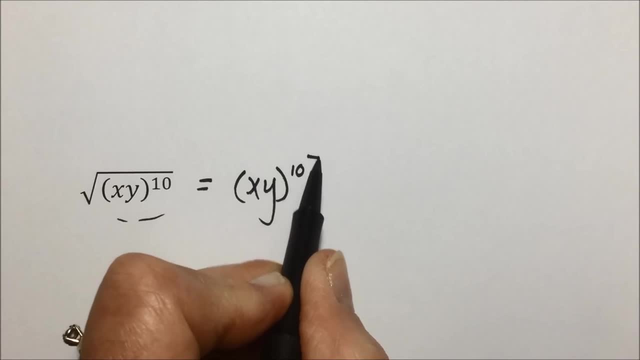 means we have x, x, y to the tenth power. Square root means it's raised to the one-half, So we've converted it to exponential Power. raised to a power we multiply 10 times one-half, 10 over 2, gives us x, y, the quantity to the fifth power.